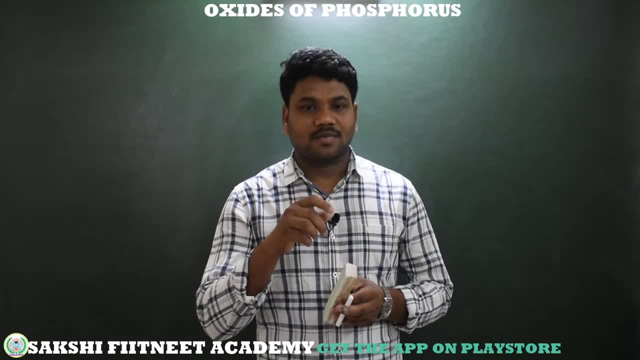 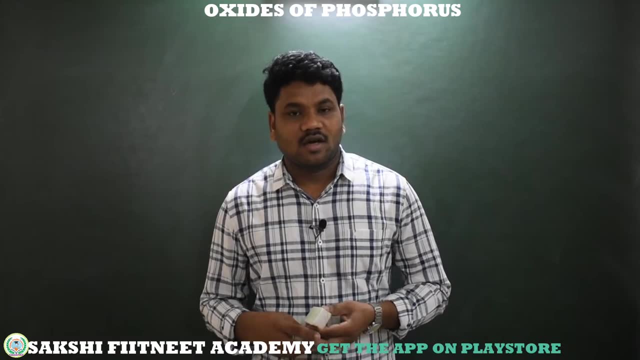 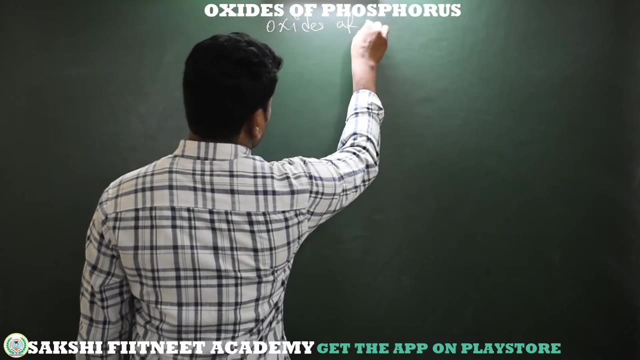 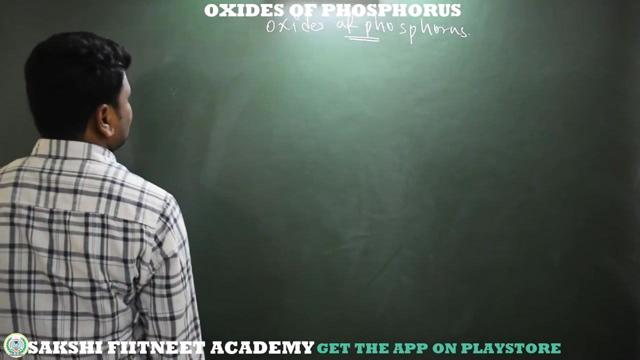 important. We observe frequent questions from these pasporous trioxide and pasporous pentoxides about their structural features. So let's begin. What are the oxides of pasporous Here, oxides of pasporous? So out of all oxides, here I am taking two major oxides. 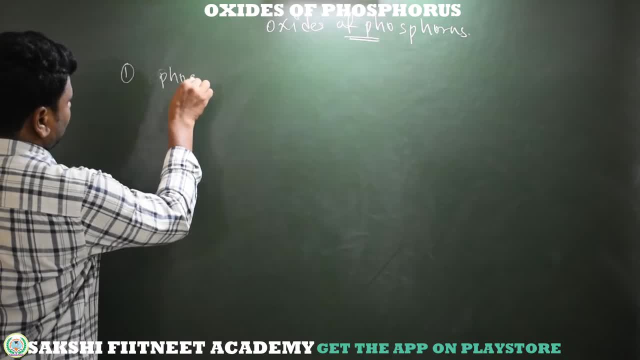 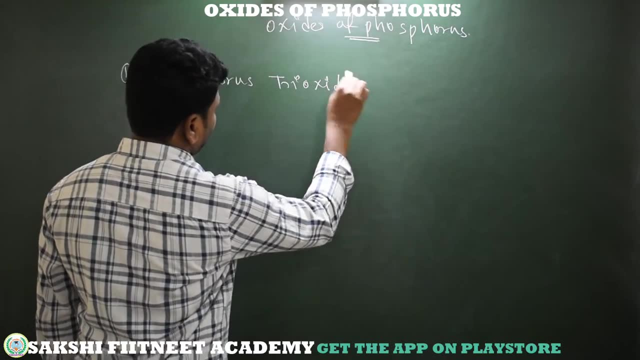 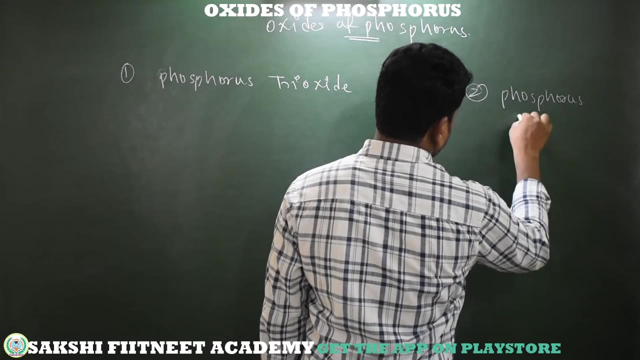 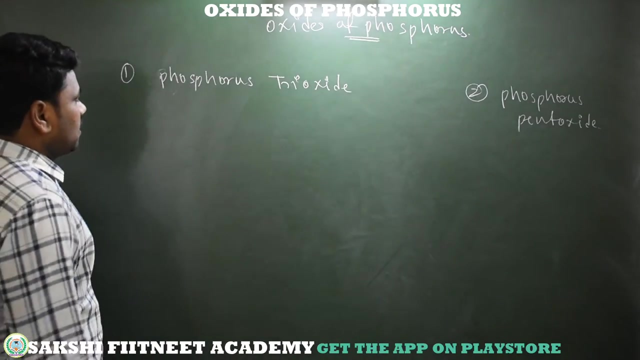 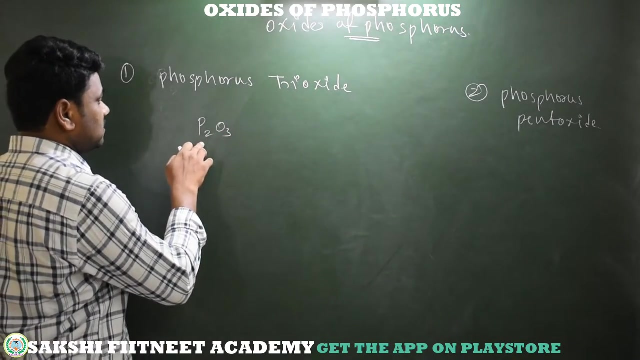 Those are that first one pasporous trioxide and second one is pasporous pentoxide. So what is the formula of pasporous trioxide? Actually, it's a P2O3 is a pasporous trioxide formula, But this is exist as P4O6.. P4O6, see here. Actually, this is not a dimer structure. 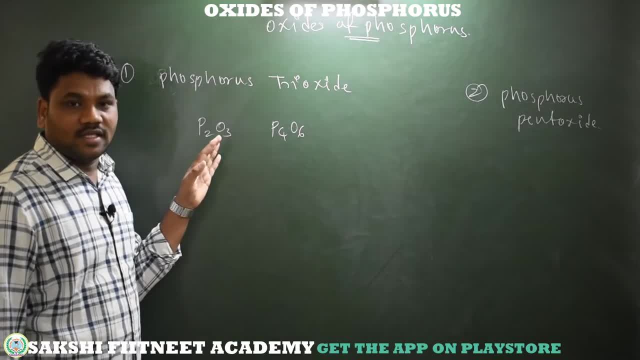 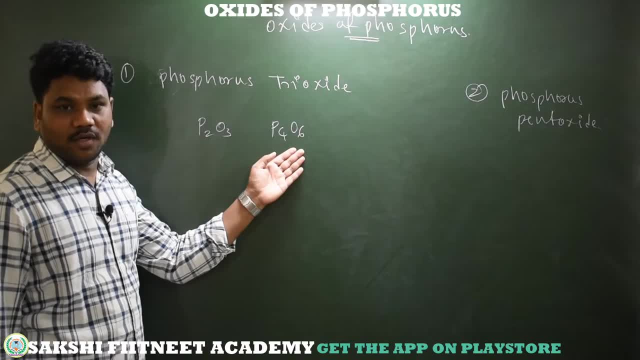 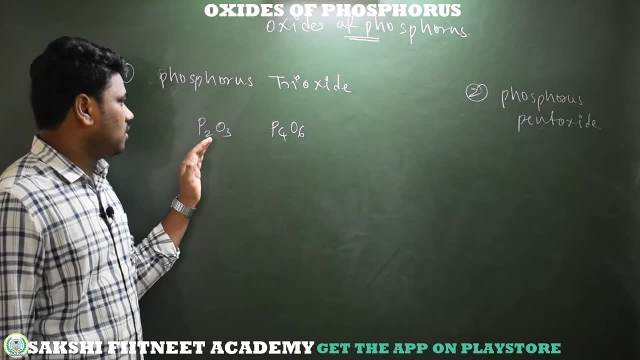 exist as a structure, So the structure existing as P4O6.. P4O6, so we can call it as a pasporous trioxide. Pasporous trioxide: Structurally it's not possible. P2O3 is structurally not. 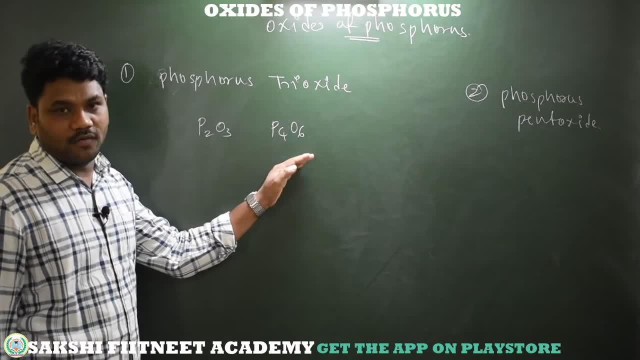 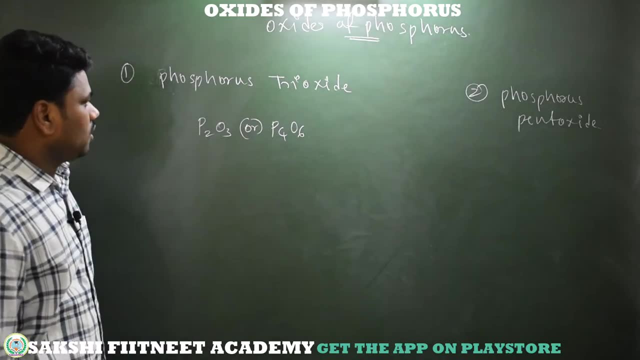 possible, So it exists in P4O6 form. P4O6 form, So we can call it as pasporous trioxide, Pasporous trioxide, So we can write P2O3 or P4O6.. P4O6. Coming to pasporous pentoxide. 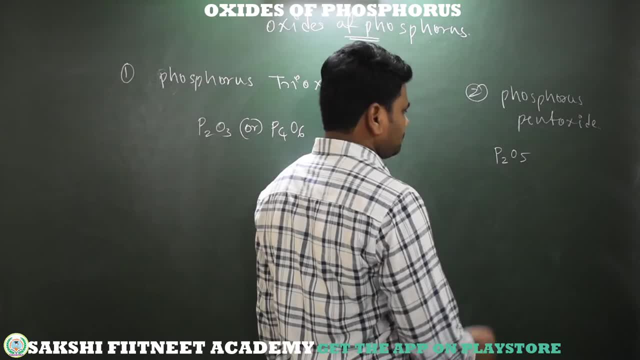 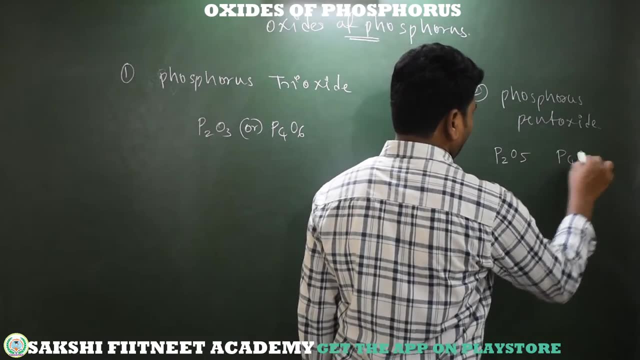 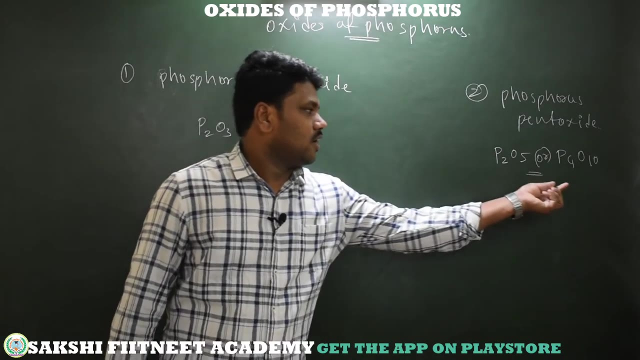 P2O5 is not structurally possible, So it exists in P4O10.. P4O10. See, here we can call it as a pasporous pentoxide. We can take formula P2O5 or P4O10.. P2O5 is structurally not possible. 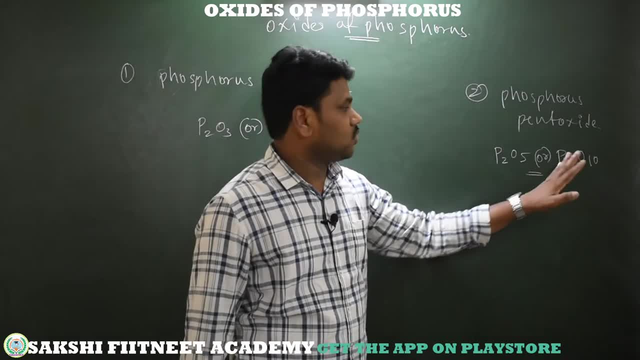 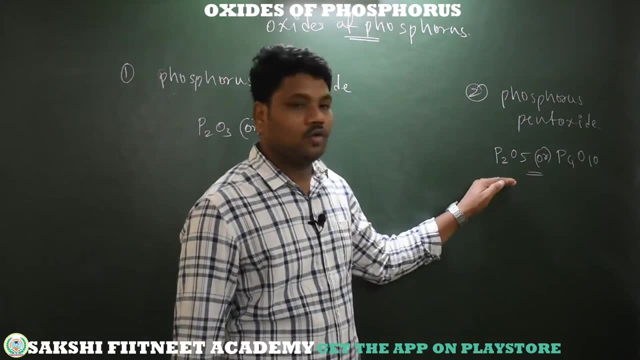 This exists as P4O10. P4O10.. So it's not a dimer form. It's not a dimer form, Just simply. the structure exists Not at P4O10.. Not at P2O5.. You just remember. So, coming to the structure of this pasporous 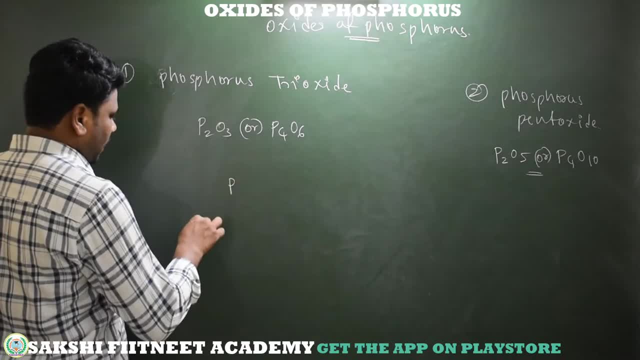 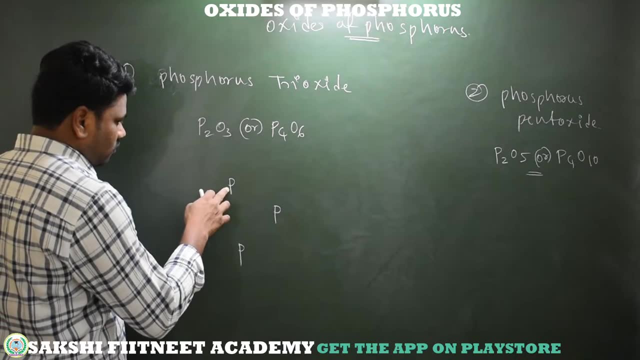 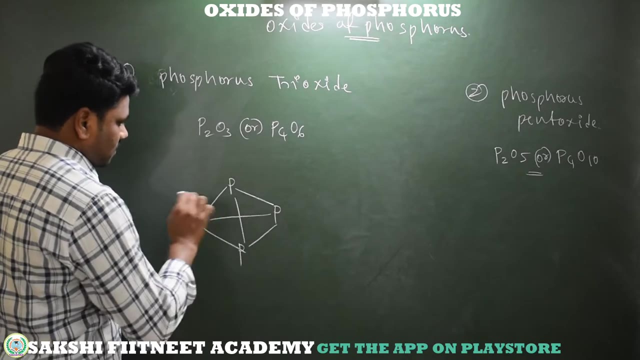 trioxide. Simply here see, we know that- white pasporous. What is the structure of white pasporous? It's a tetragonal manner, So each pasporous bonded to pasporous to pasporous, Each pasporous actually bonded to three other pasporous atoms, Three other pasporous atoms. 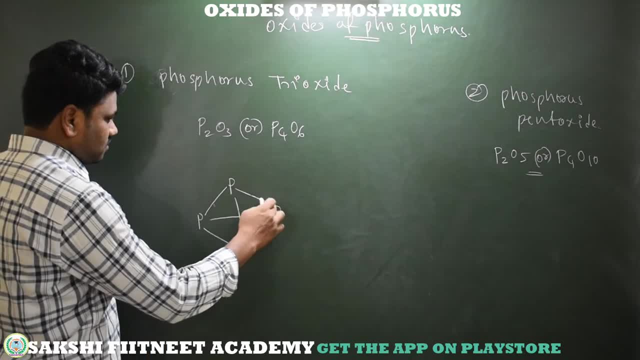 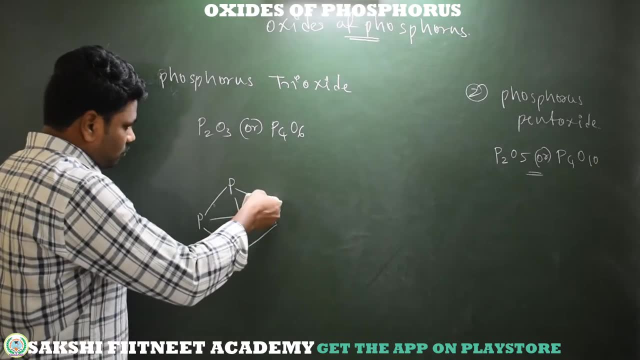 See here these pasporous bonded to 1,, 2,, 3.. And these pasporous bonded to 1,, 2, 3.. The two other three pasporous atoms You just break, these pasporous to pasporous bond. 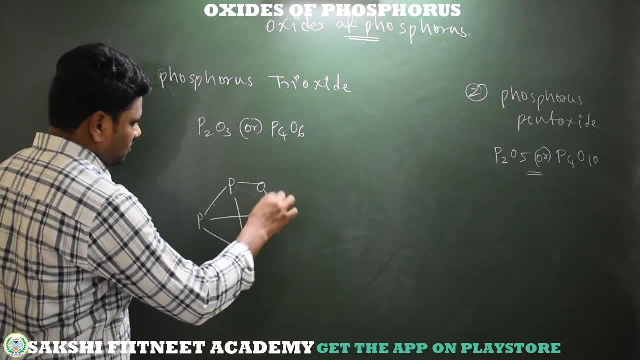 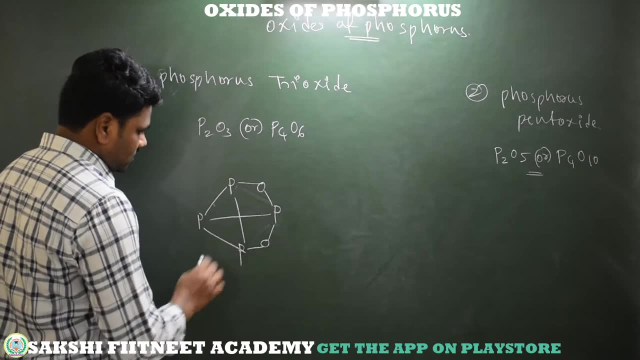 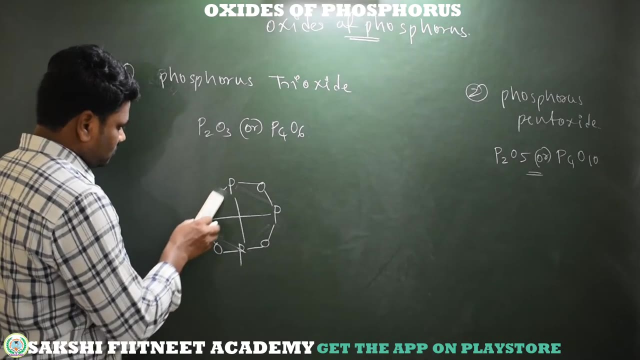 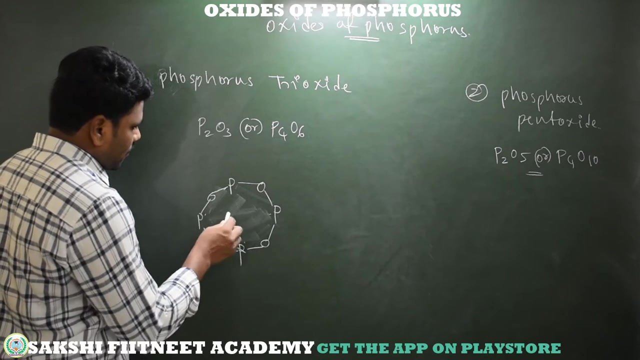 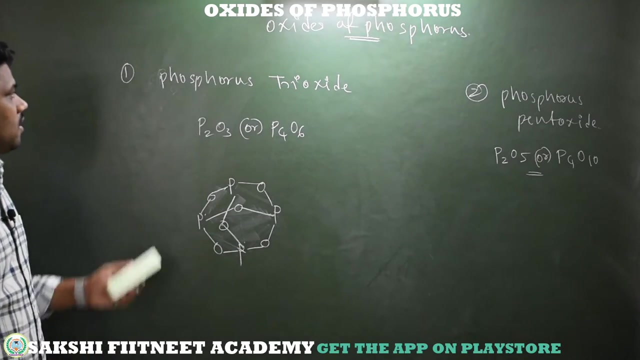 And make a bridge bond through oxygen, Make bridge bond to oxygen- See here. I am just making a bridge bond through oxygen, See here. And now I am just breaking the two pasporous bonds, See here. so this is the structure of. 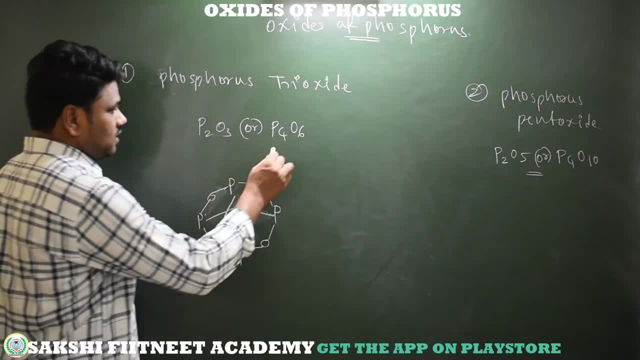 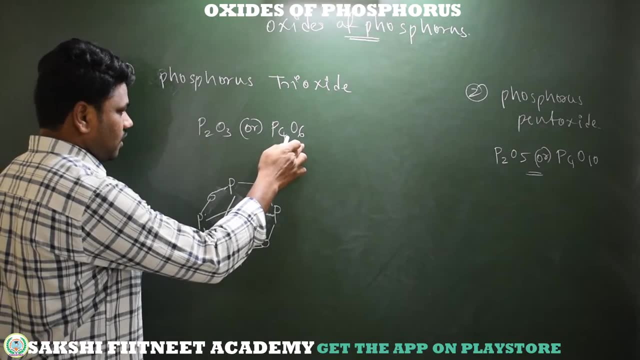 phosphorus trioxide with this formula. with this formula, see here 1,2,3,4, 4 phosphorus atoms and how many oxygens are there. we have 1,2,3,4,5,6, 6 oxygen atoms are there. 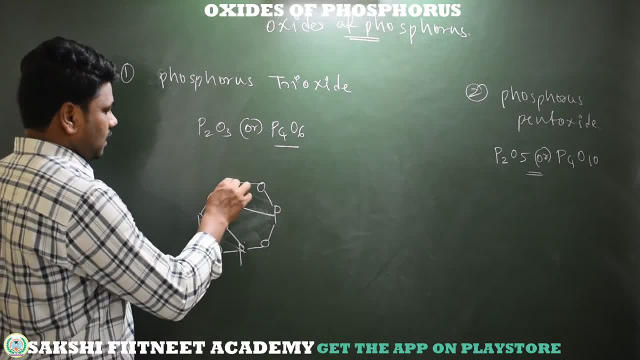 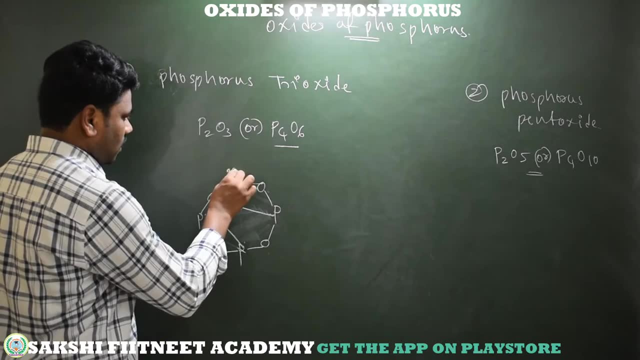 now coming to the geometry of each phosphorus. see here: this is the phosphorus which, having a 3, bonds with a 3 bridged oxygen atoms, and here we have 1 lone pair. we have 1 lone pair coming to this phosphorus, 1,2,3. 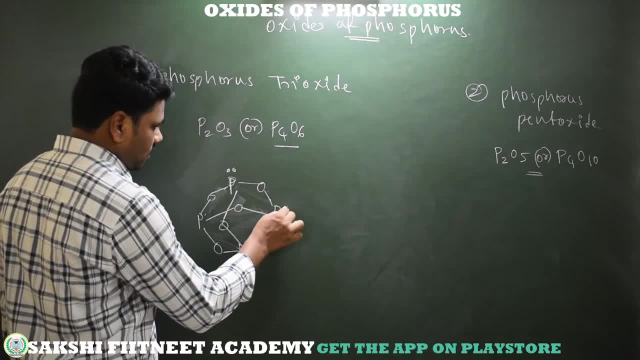 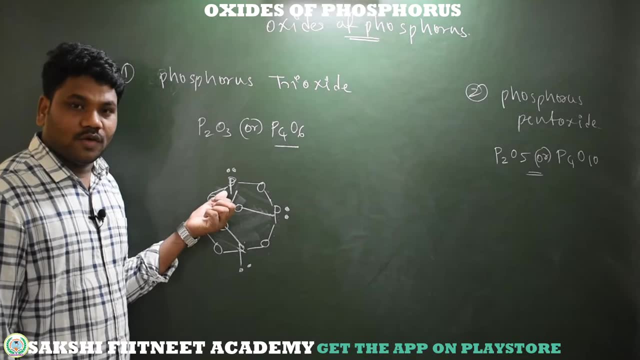 bridged bonded with a 3 bridged oxygen atoms. and here we have 1 lone pair. coming to this phosphorus- same. coming to this phosphorus- same. we know that phosphorus belongs to 5th group. that means 3 unpares, 1 lone pair. 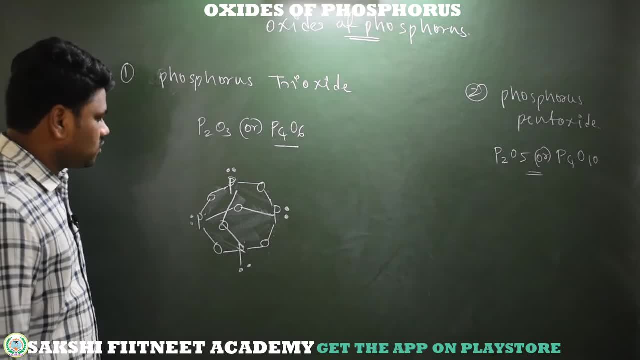 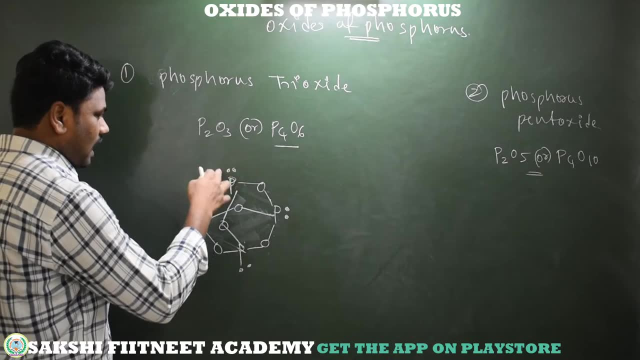 see here 1 lone pair and 3 unpares. so what is the hybridization of each phosphorus in this phosphorus trioxide? 1,2,3, 4, 2 electrons are as a pair. that means hybridized 1,2,3. 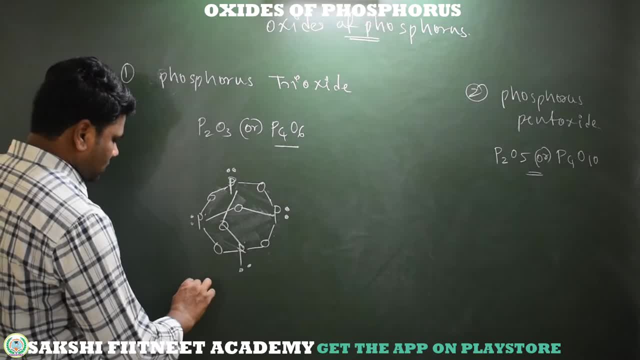 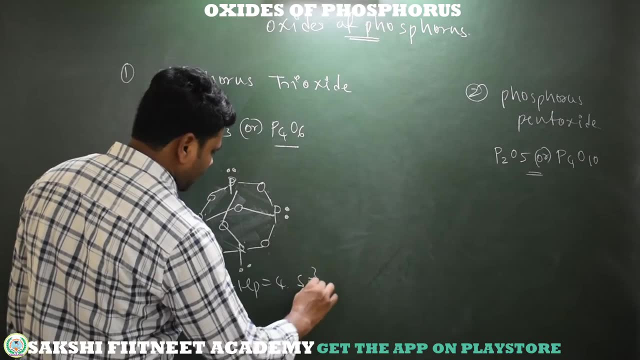 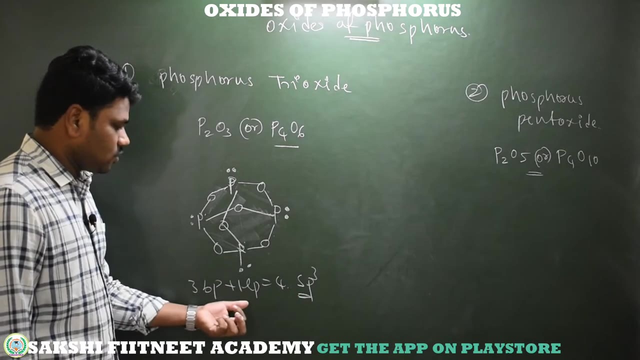 4, that 4 are existing as 3 bond pairs plus 1 lone pair. that is equal to 4. obviously it's a sp3 hybridized. sp3 hybridized. and what about the geometry? sp3 hybridized, 3 bond pairs, 1 lone pair. 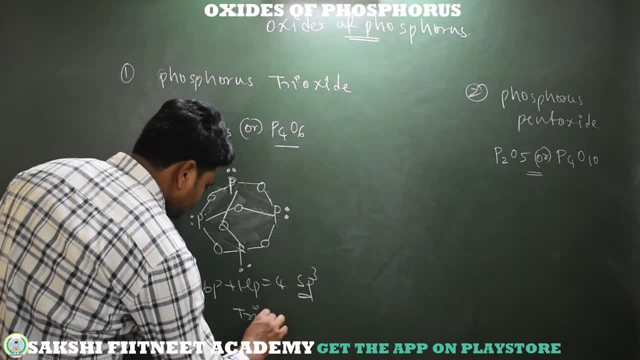 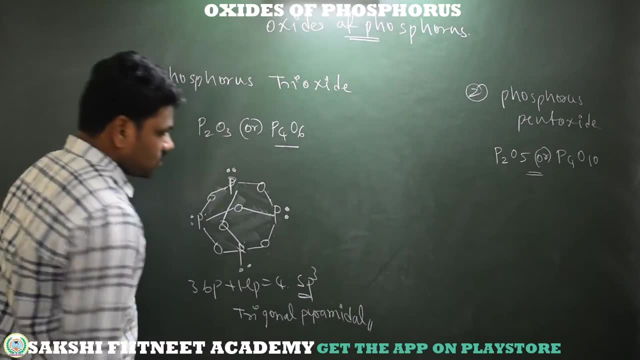 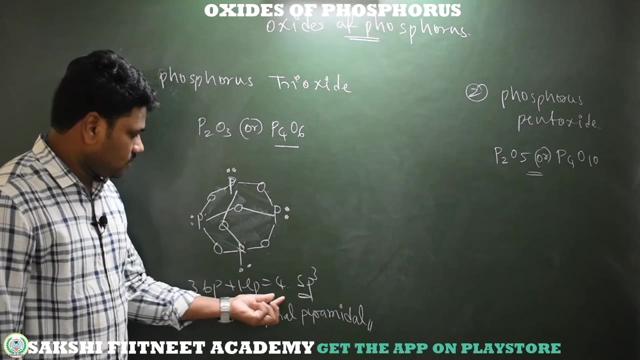 so obviously it's a trigonal, trigonal, trigonal pyramid, trigonal pyramid. this is the geometry of the geometry of phosphorus in this phosphorus trioxide: 3 bon pares, 1 lone pair. it's equal to 4 sp3 hybridization with 3 bond pairs, 1 lone pair. 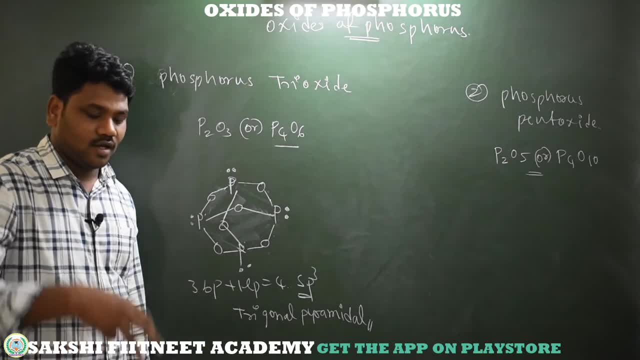 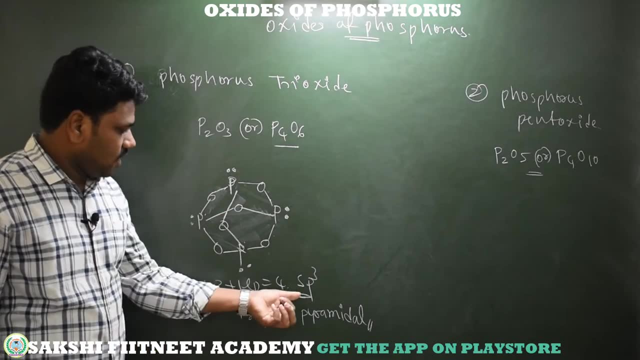 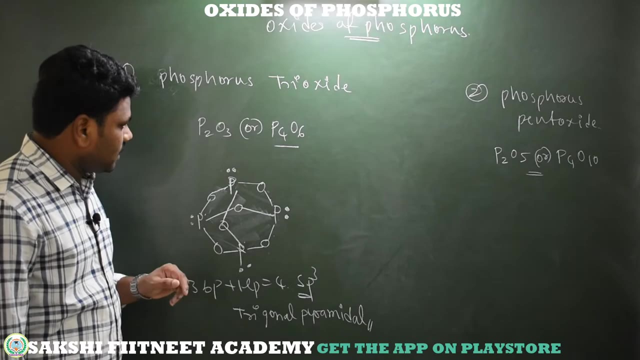 it's become trigonal pyramid, like it's a ammonia: 3 bonds towards down, like a pyramid: 1 lone pair is towards upside. so each phosphorus experiencing sp3 hybridization trigonal pyramidal coming to a Sigma bonds coming to Sigma bonds and number of bridged oxygens: number of bridged: 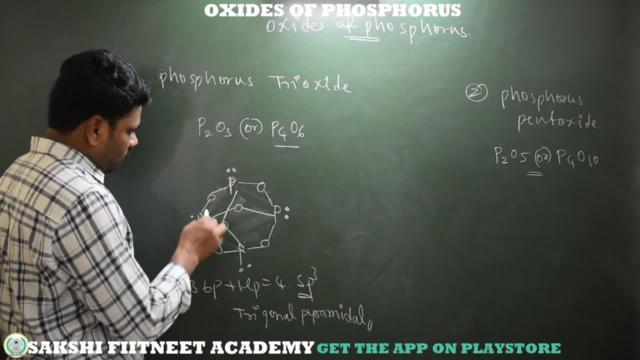 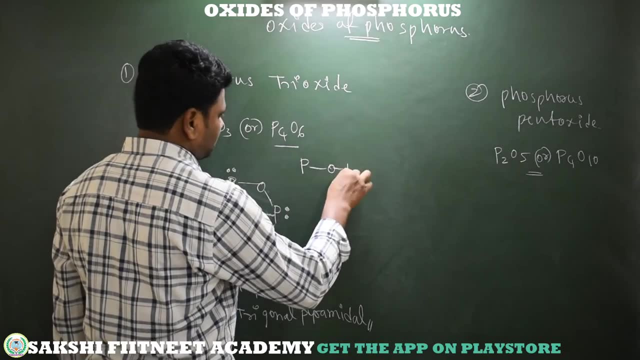 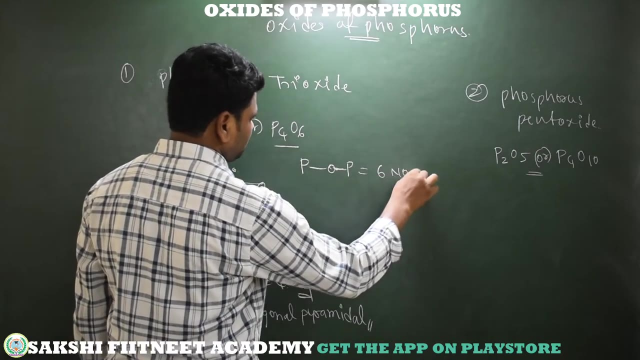 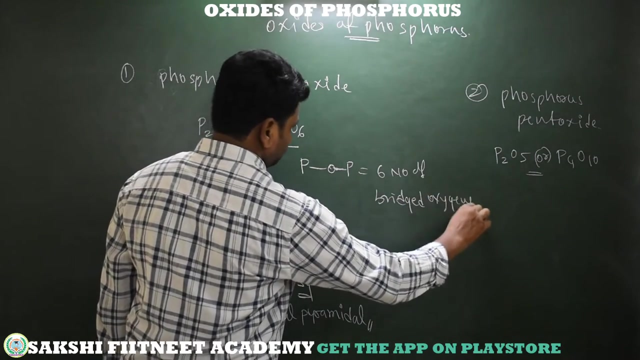 oxygens. see here we have one, two, three, four, five, six, six oxygens are there. we have six bridged oxygens, that is, phosphorus to phosphorus through oxygen, so this is called a bridged oxygens. how many are there? these are six, number of bridged oxygens we have. so now coming. 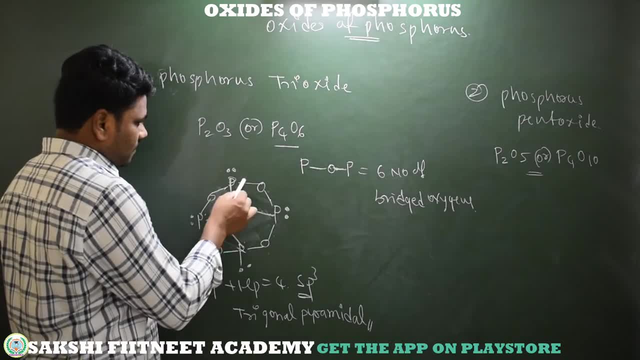 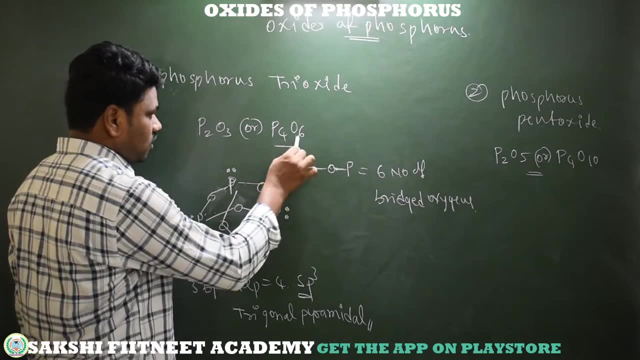 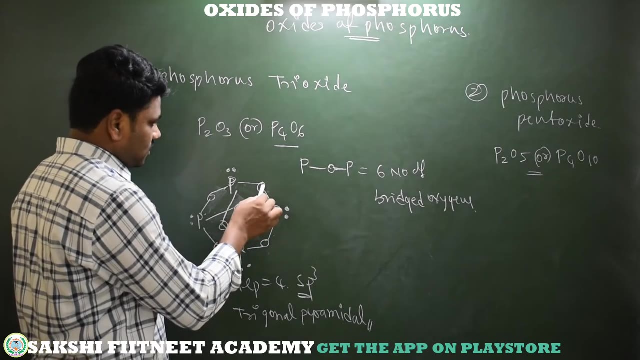 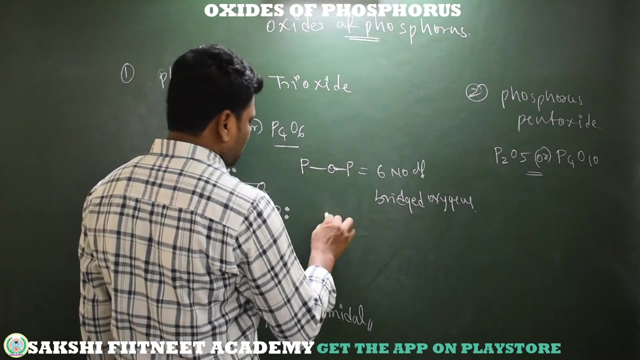 to total number of Sigma bonds. see here: one, two, three, four, five, six, seven, eight, nine, ten, eleven, twelve. simply here, each oxygen gives two Sigma bonds. each oxygen gives two Sigma bonds towards two phosphorus atoms. see here this oxygen: one, two, three, four, five, six, six, seven, eight, nine, ten, eleven, twelve. so total we have twelve Sigma bonds. we have twelve. 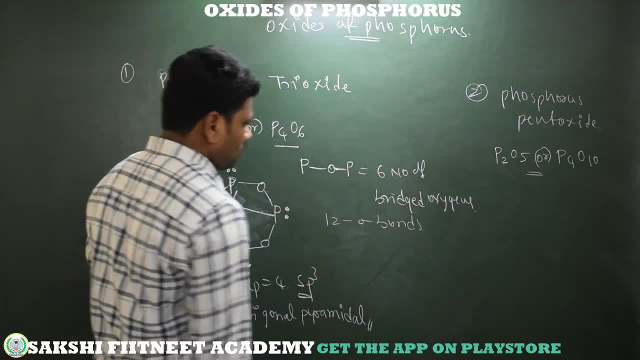 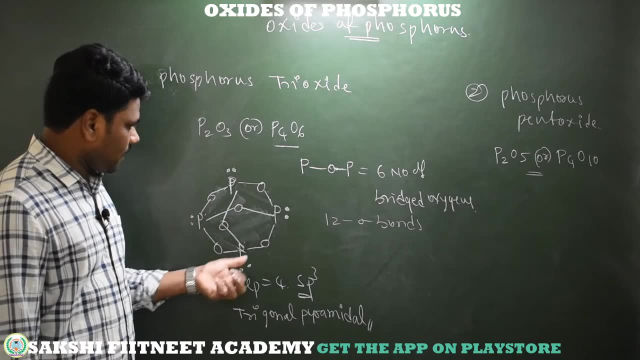 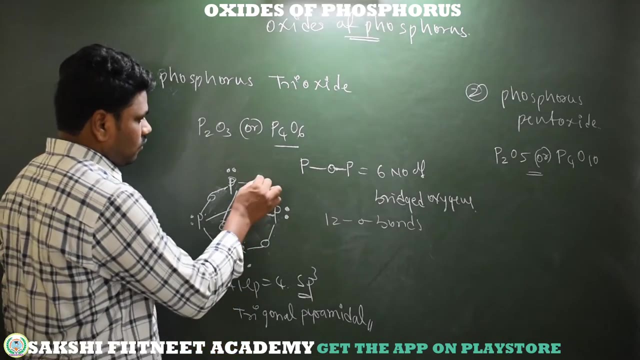 six, twelve Sigma bonds. coming to lone pairs. coming to lone pair. see here each phosphorus giving one lone pair one, two, three, four. plus each oxygen shows two lone pairs, two bond pairs. see here two bones pairs and here we have other two lone pairs because oxygen belongs. 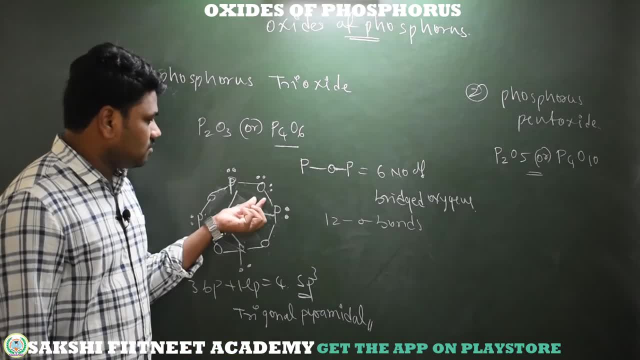 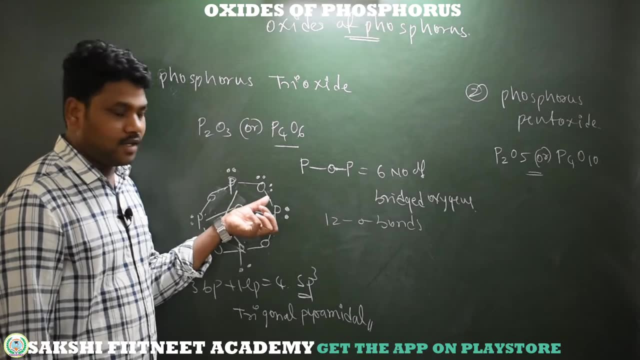 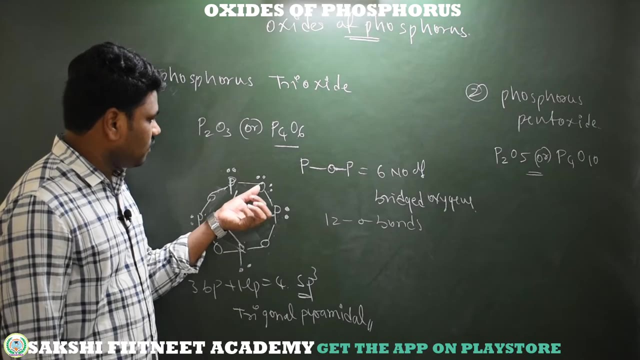 to 6th group. that symbolizes wislapping atmosphere. remember this does not happen again. 3, 1, not six valency electrons exist as two lone pairs and two unpairs. These two unpairs are involved in a sigma bond formation that is covalent bond formation. So around each oxygen we have two. 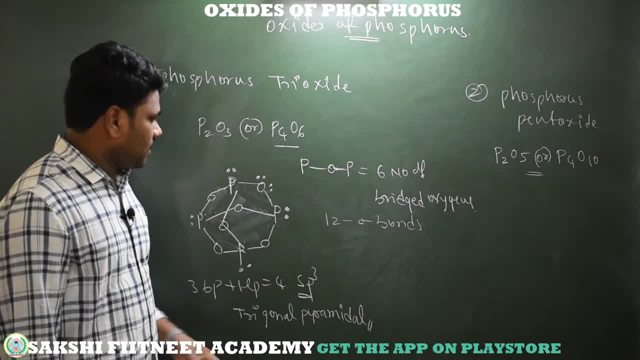 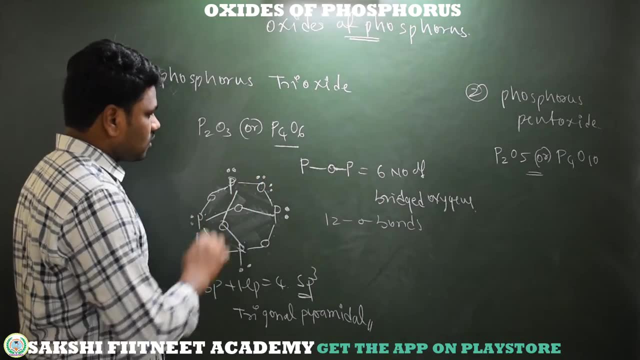 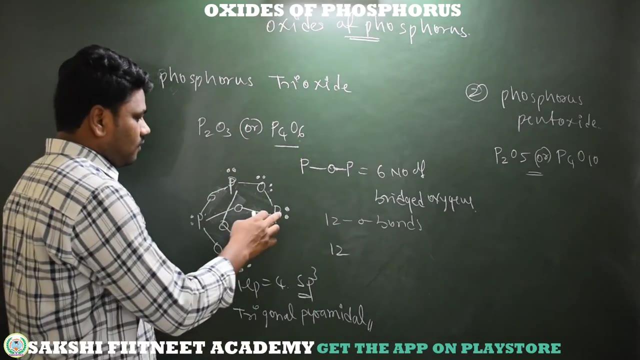 lone pairs and two bond pairs. So total number of lone pairs in this phosphorus trioxide: see here each oxygen shows two lone pairs. that means here we have six oxygens, six into two, that is twelve. twelve lone pairs from six oxygens and four lone pairs from four phosphorus atoms: one, two, three. 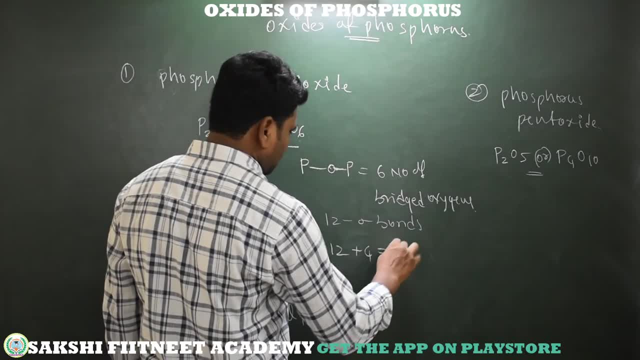 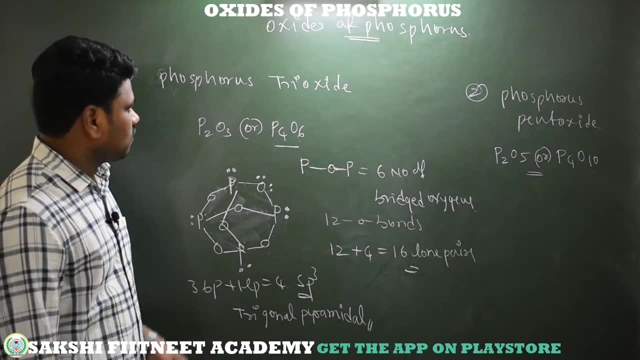 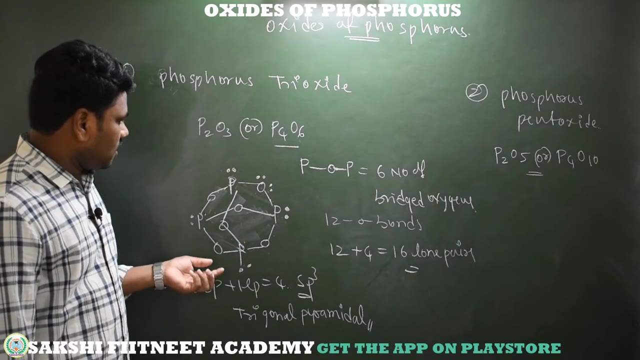 four, Four lone pairs from four phosphorus atoms. that is equal to sixteen lone pairs. Here we have total, sixteen lone pairs. This is a structure of phosphorus trioxide. Simply, here, each phosphorus bonded to three oxygen bridge atoms and here the total, all the four phosphorus each phosphorus. 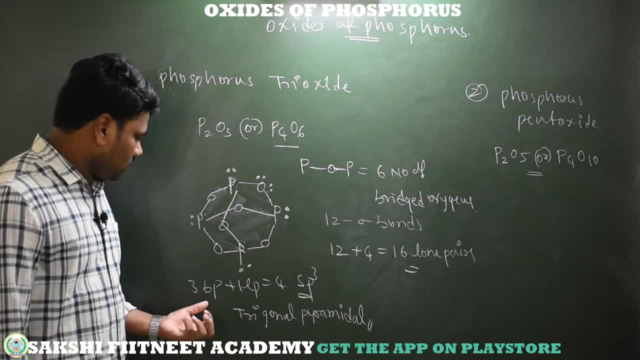 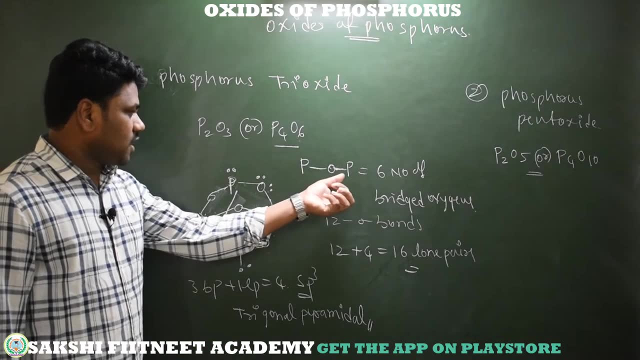 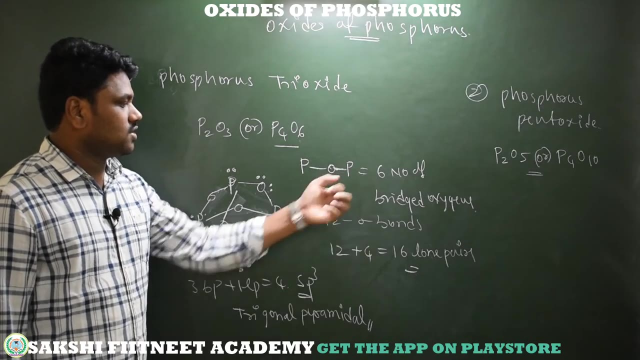 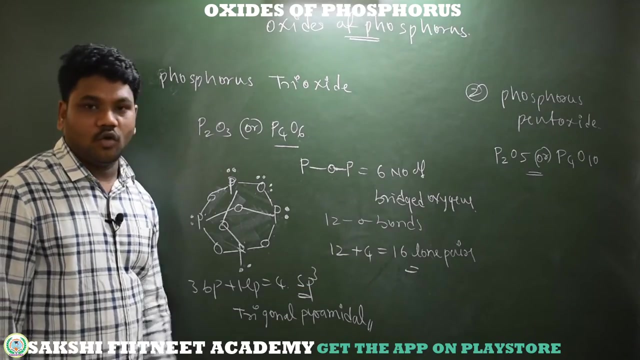 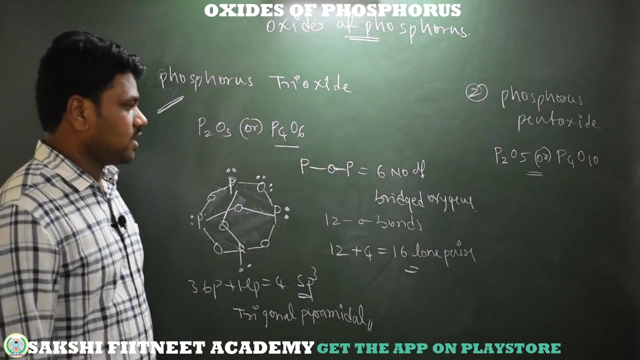 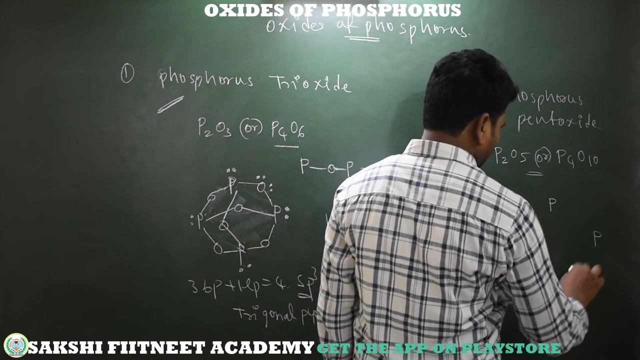 experience. Let us switch the puppy. What about the loan para 16 lone pairs? So this is a structure of phosphorus trioxide transfer, The see here structure of phosphorus pentoxide, same here. take four phosphorus atoms which are like present in a white phosphorus, white phosphorus like a tetragonal. now each phosphorus 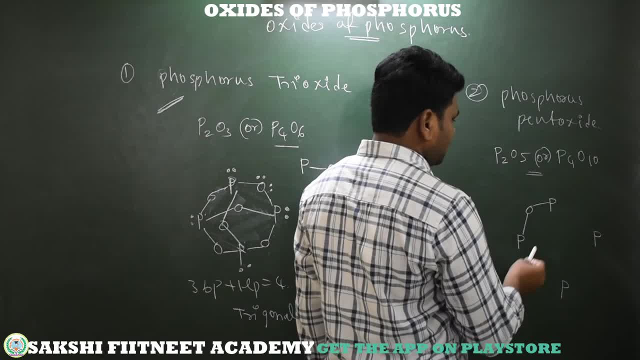 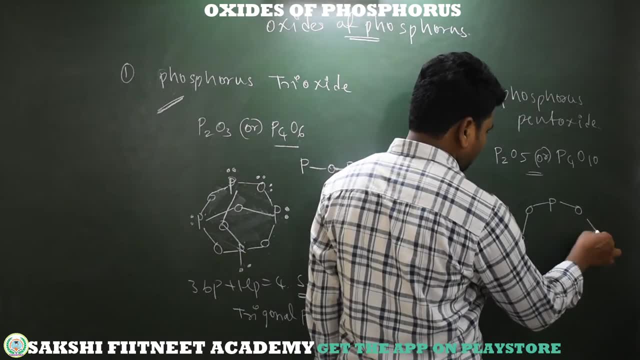 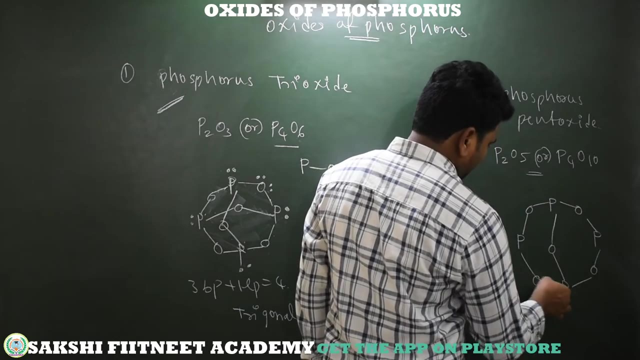 same, like phosphorus trioxide. so each phosphorus having a three oxygen bonds. see here this phosphorus with this oxygen, with this oxygen and here with this oxygen. now coming to this phosphorus, bridged oxygen directly you can draw. see here each phosphorus having a three. 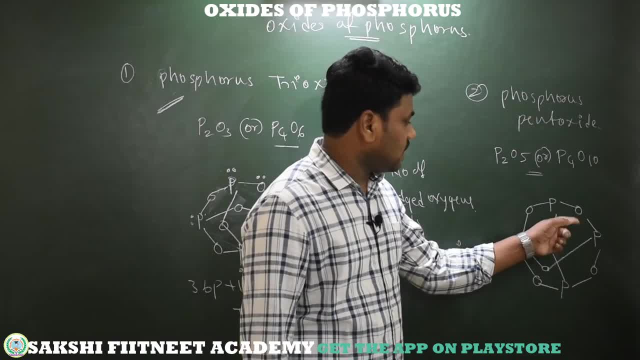 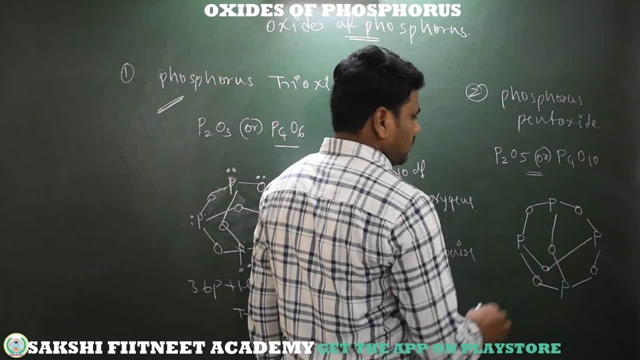 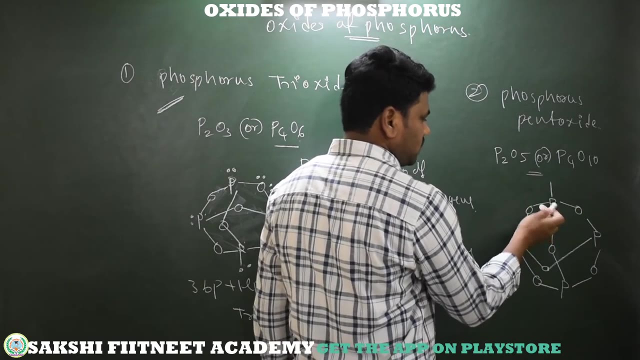 oxygen bonds, three oxygen bonds. those oxygens are existing as bridged atoms, bridged atoms. so here we have total six bridged oxygen atoms and remaining four oxygens are forming a coordination bond with this phosphorus, coordination bond with this phosphorus. so we can represent one. 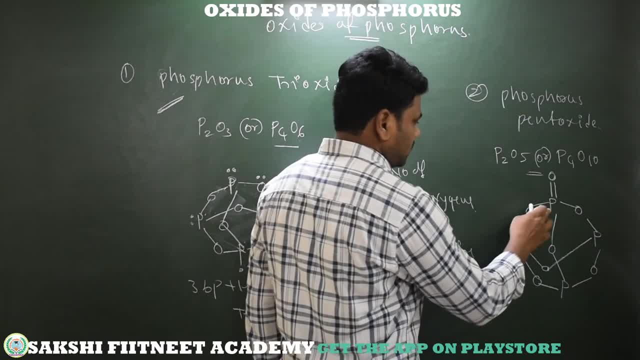 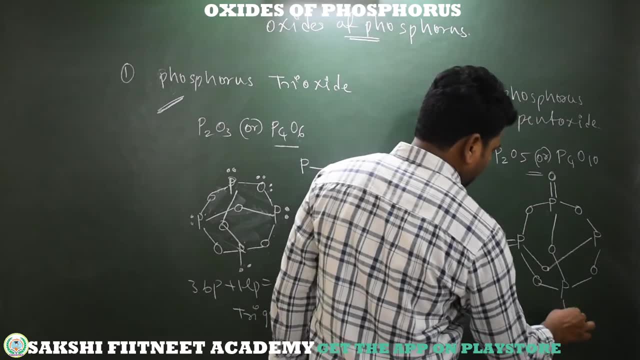 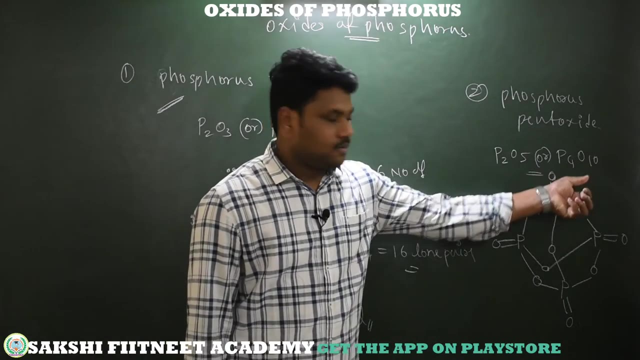 sigma bond, one pi bond, one sigma bond, one pi bond with this phosphorus, phosphorus bonded to oxygen. one is sigma, one is pi. now, here we have other oxygen, here we have other oxygen and here we have other oxygen. see here what is the formula: it's a p4 o10. now, one, two, three, four, it's p4 o10, we have. 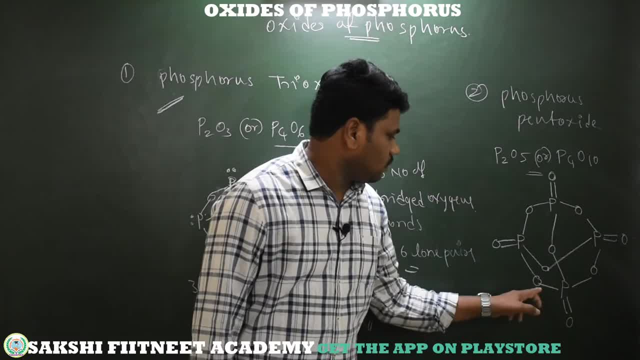 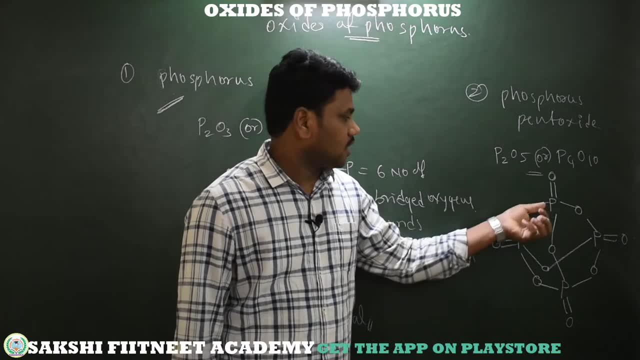 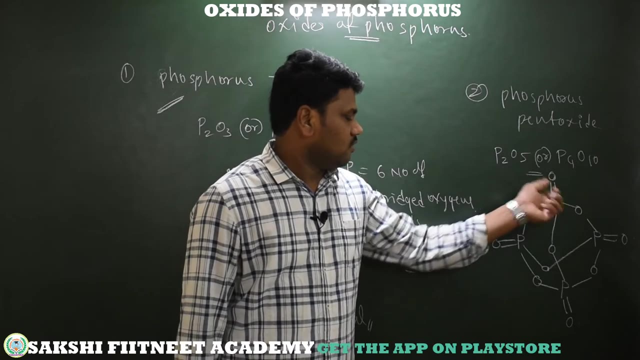 six bridged oxygen atoms: one, two, three, four, five, six and remaining oxygens are existing as like a carbonyl oxygen, here phosphorus instead carbon. here we have a phosphorus double bond, see here phosphorus to oxygen. one sigma bond, one pi bond. one sigma bond, one pi bond. now coming to, 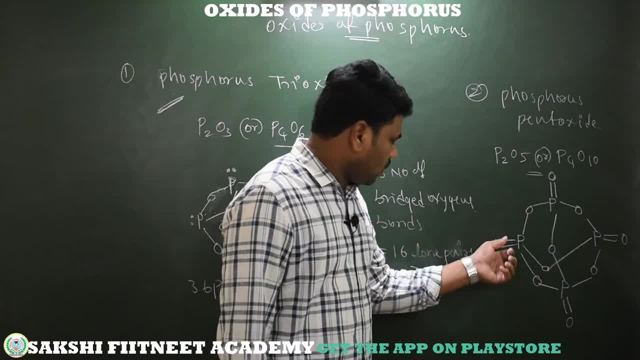 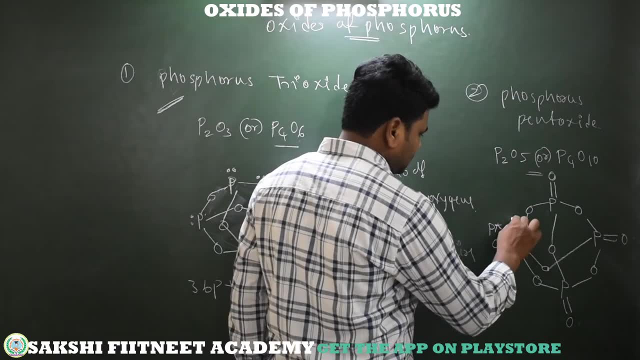 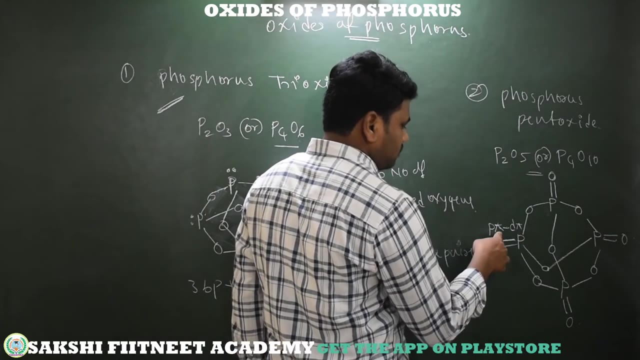 this sigma bond and pi bond. see here this pi bond due to the p pi orbital. you can see here this pi bond due to the p pi orbital: p pi 2. this is d pi, not p pi, not a p pi. see here this is a bond due to the p orbital, pi electron. 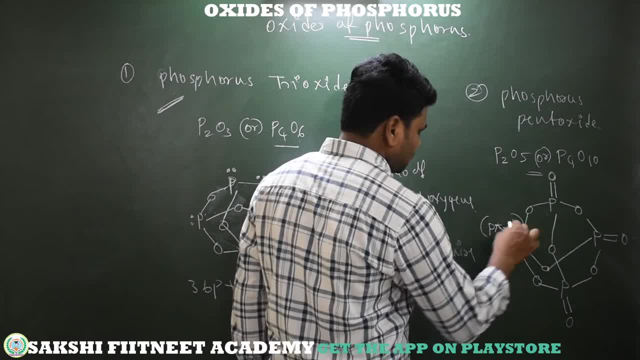 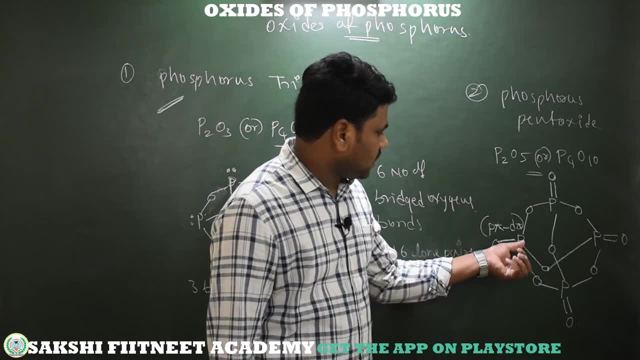 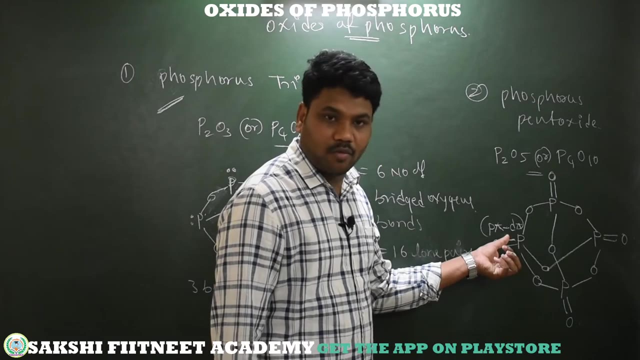